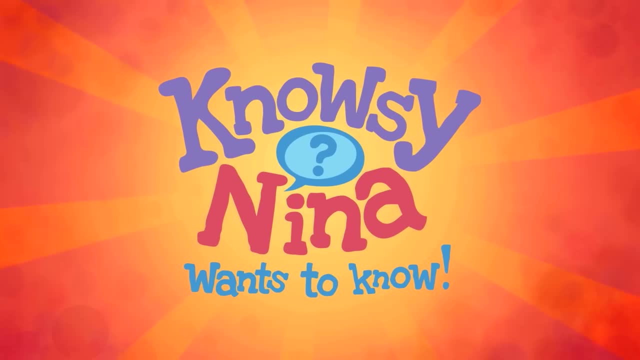 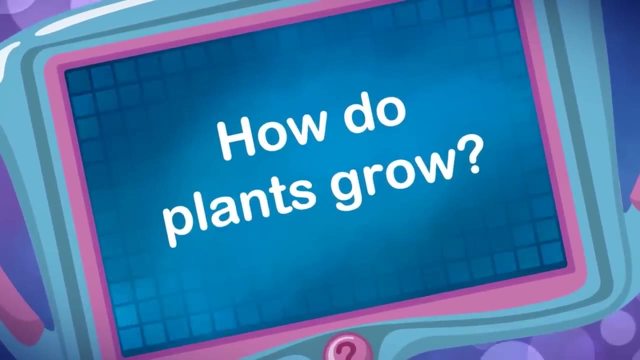 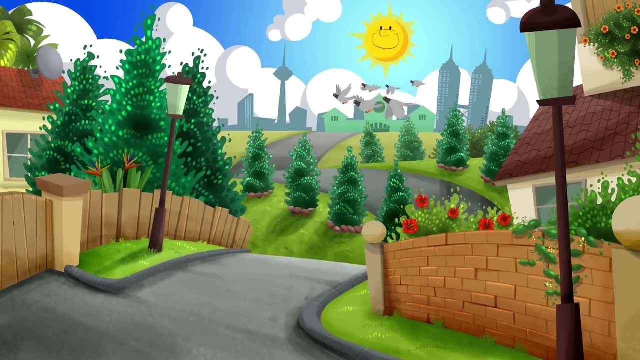 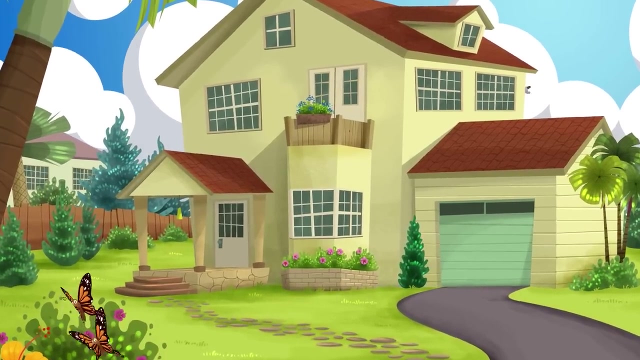 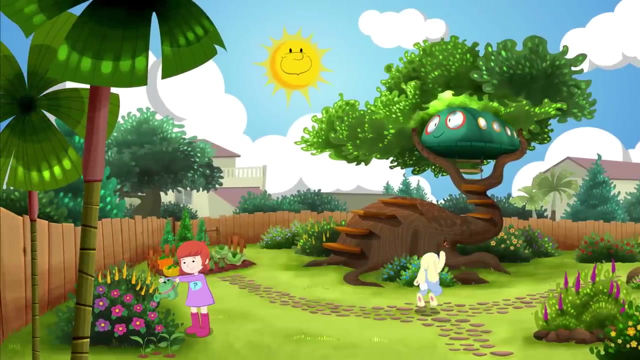 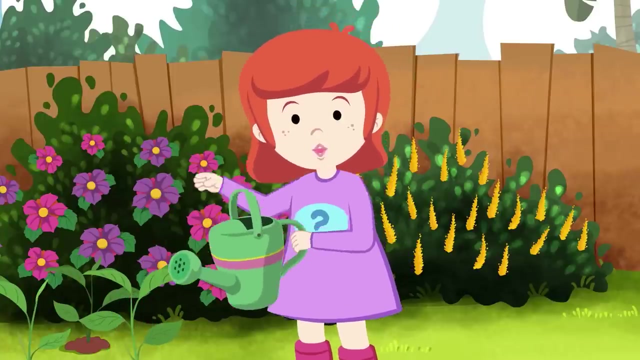 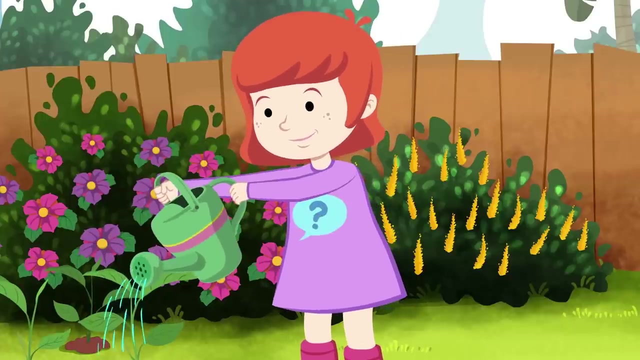 In a little town, in a little house, lives a little girl called Nosy Nina. Let's see what she's up to today. Hello there, Nosy Nina. Hello there, Mr Voice. What are you doing? The plants are thirsty, so I'm giving them a drink. 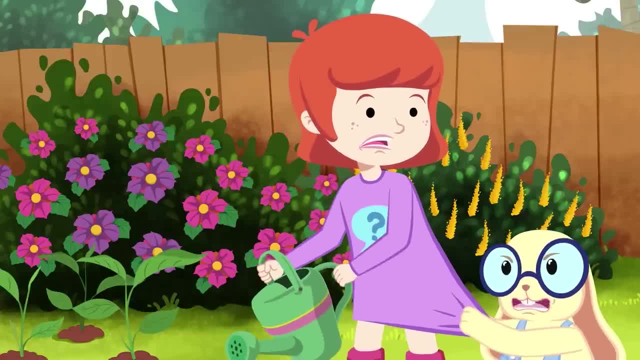 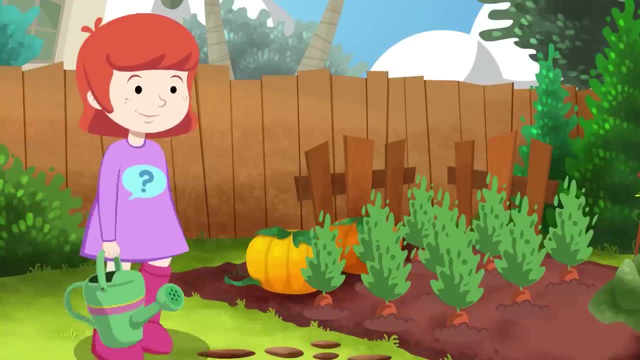 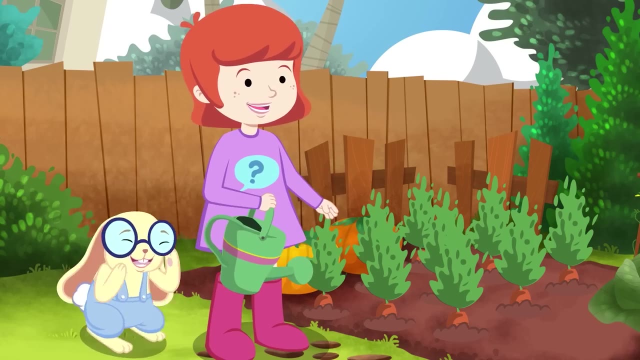 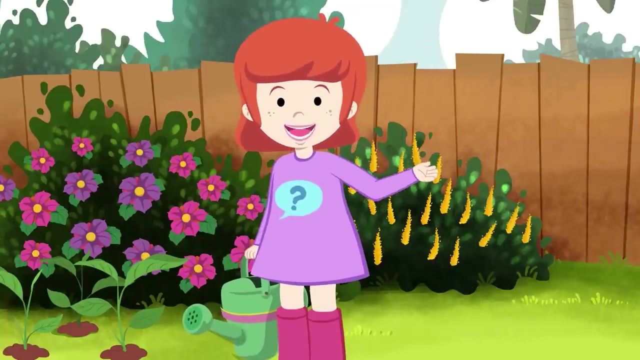 Don't worry, Smarty Pants, Of course I'll give your carrots a drink too. That's so thoughtful of you, Nina. Now all your plants will grow healthy and strong. Yes, I love to watch the baby plants grow into big adult plants. 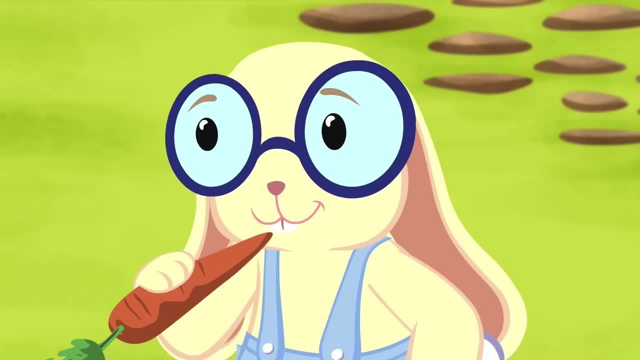 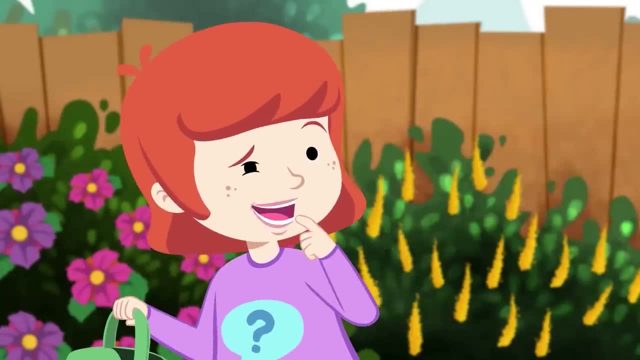 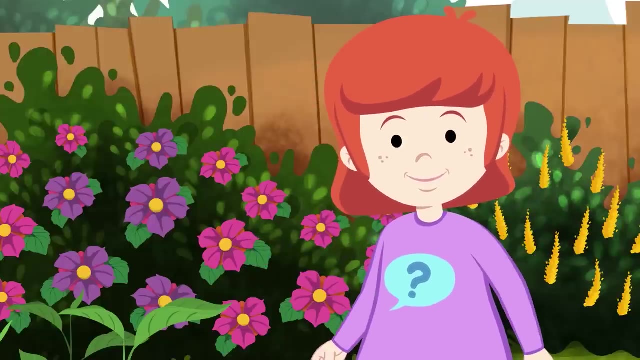 They grow so fast. Beep, beep, beep. How do they grow? I'm not sure, Smarty Pants, Maybe Mr Voice knows. Mr Voice, how do plants grow? I thought you'd never ask. Let's take a look at the Knowledge Pad. 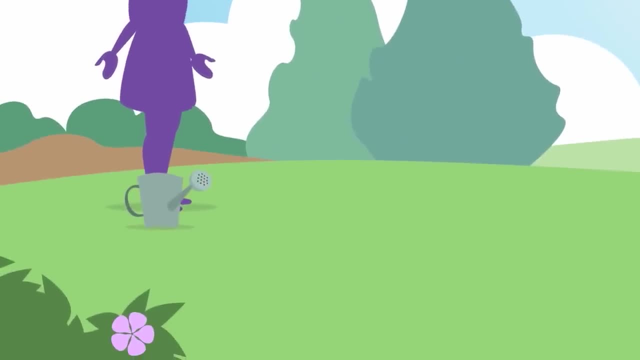 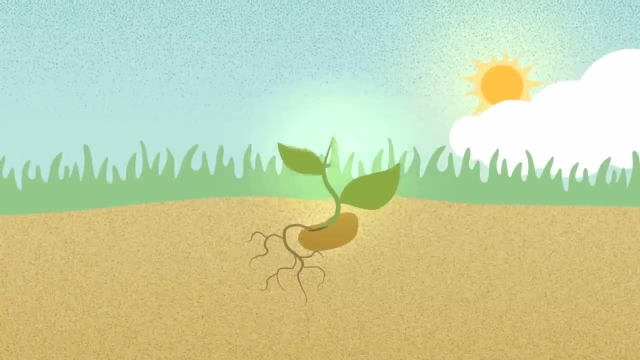 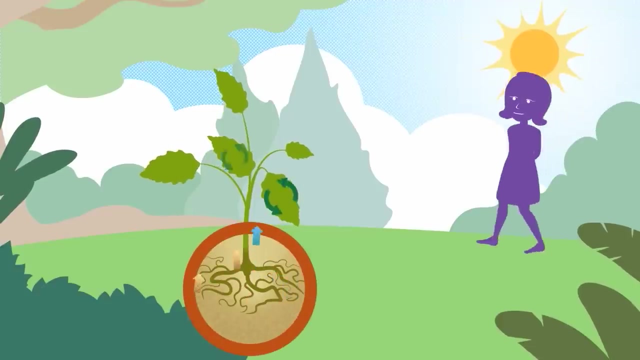 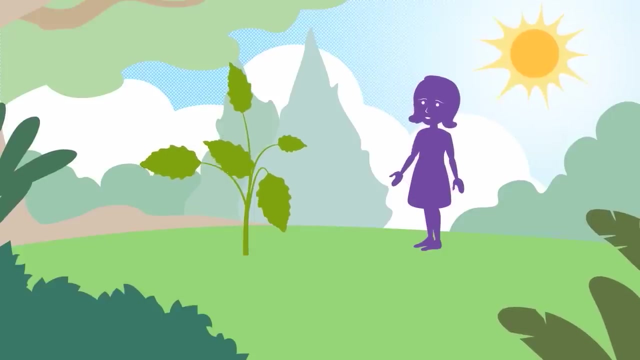 The Knowledge Pad. Well, Just like you and me, a little seed needs water, food and sunlight to grow healthy and strong. Plants are special because they make their own food, and we help them do this When we breathe. the air we breathe out is used by the plants to make food for them to eat. 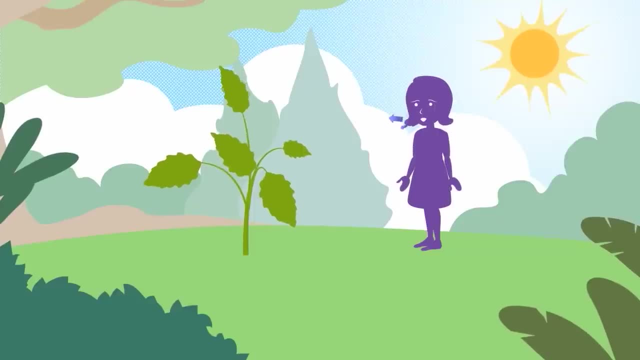 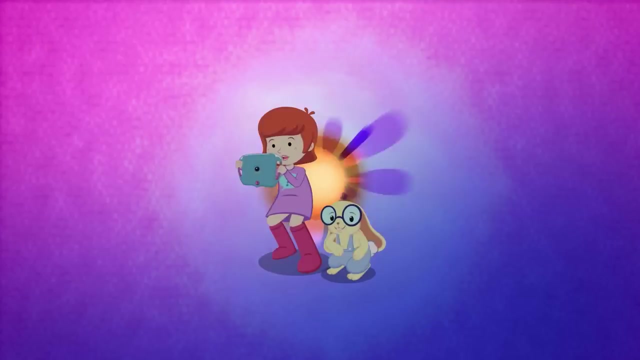 Plants also take the air we breathe out and turn it into fresh new air for all of us to breathe. So we need plants to live and they need us to grow. And that's how plants grow. Wow. So now I know. 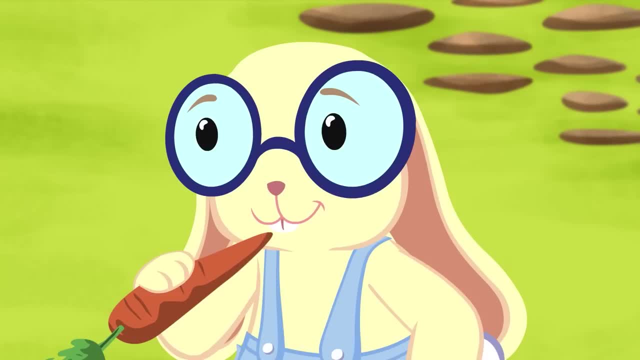 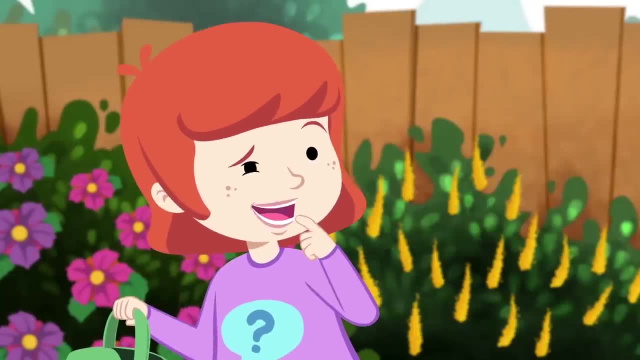 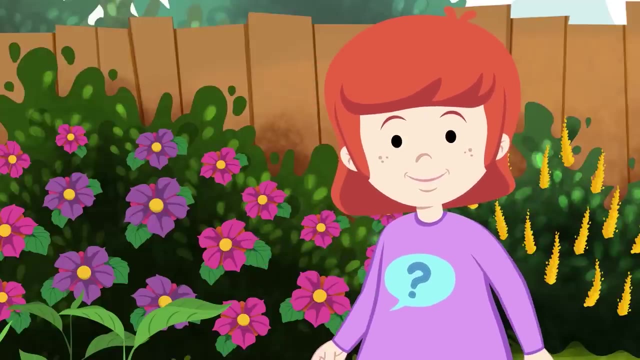 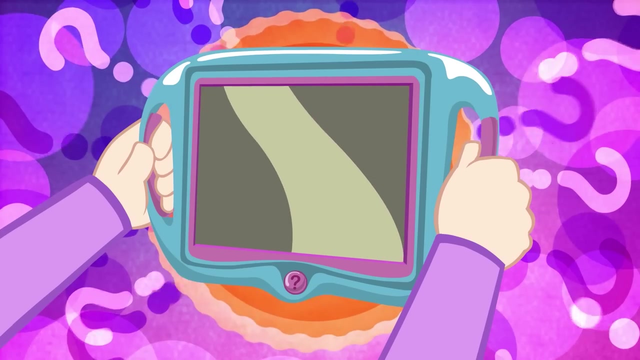 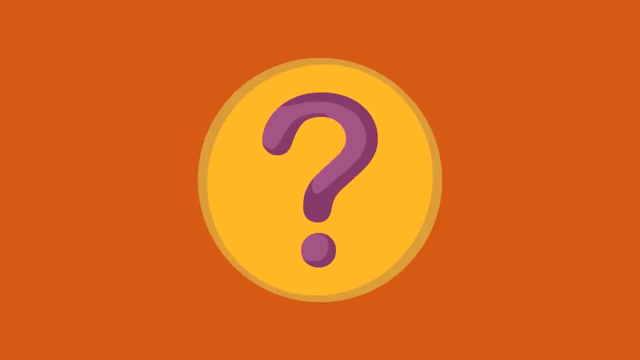 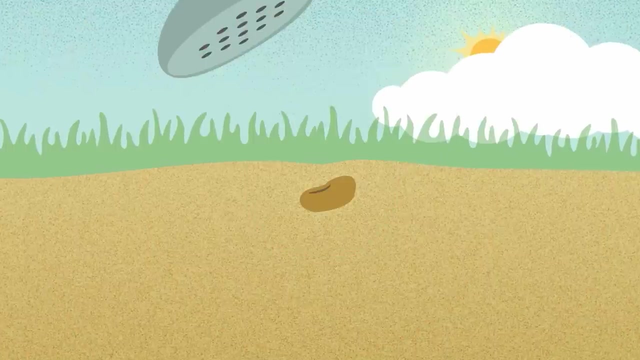 They grow so fast? how do they grow- I'm not sure- smarty pants? maybe mr voice knows. mr voice, how do plants grow? I thought you'd never ask. let's take a look at the knowledge pad. well, just like you and me, a little seed needs water, food and sunlight to grow healthy. 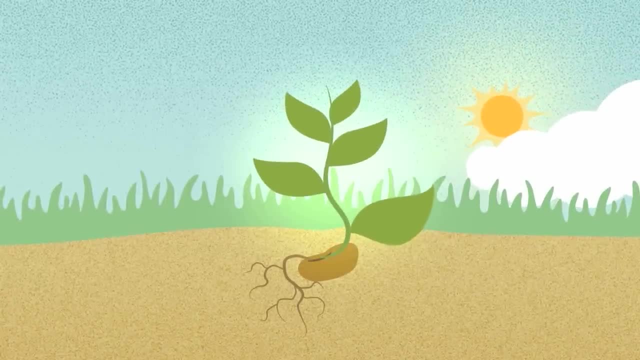 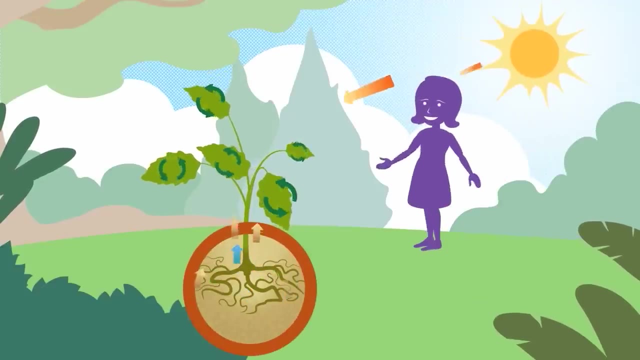 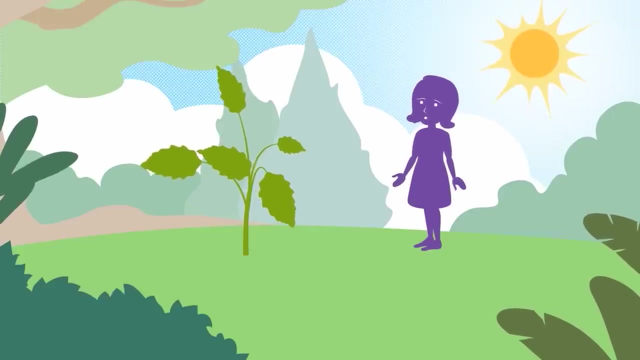 and strong plants are special because they make their own food and we help them do this when we breathe. the air we breathe out is used by the plants to make food for them to eat. plants also take the air we breathe out and the air we breathe out to make food for them to eat. plants also take the air we breathe out and. 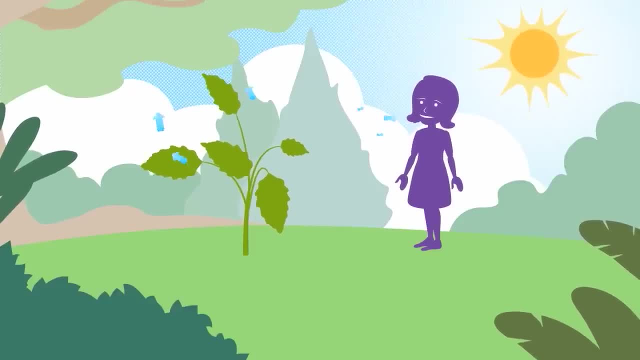 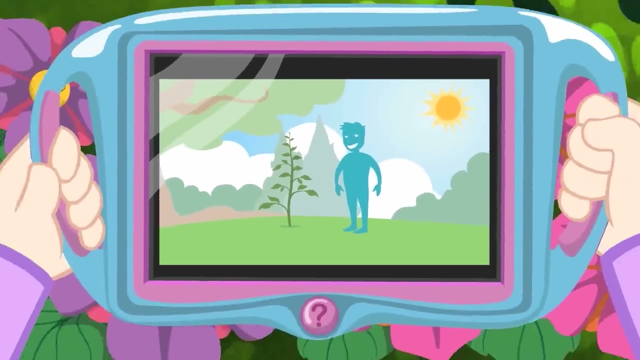 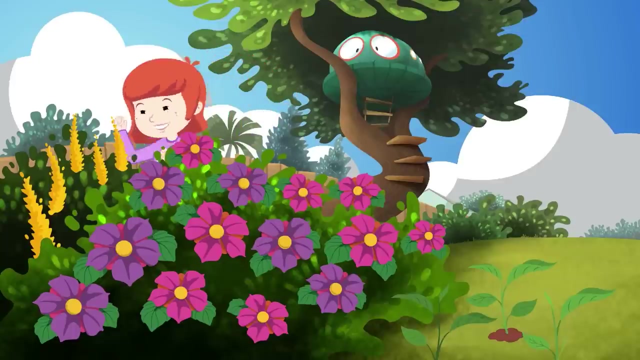 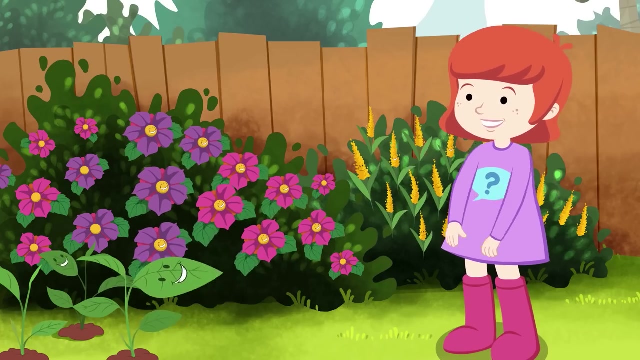 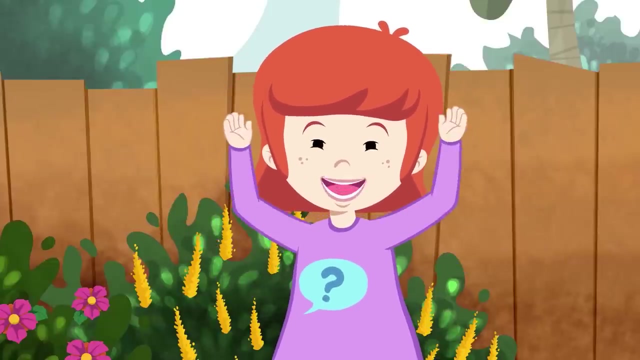 turn it into fresh new air for all of us to breathe. so we need plants to live and they need us to grow, and that's how plants grow, and they need us to grow, and that's how plants grow. wow, so now I know. so plants are very important to all of us because they make clean air for us to. 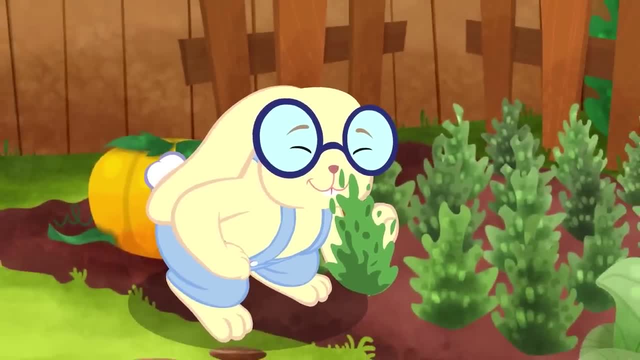 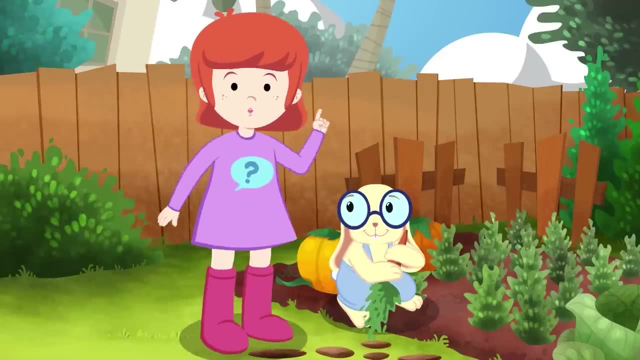 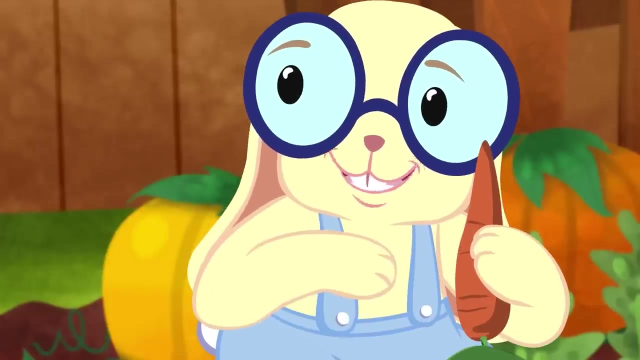 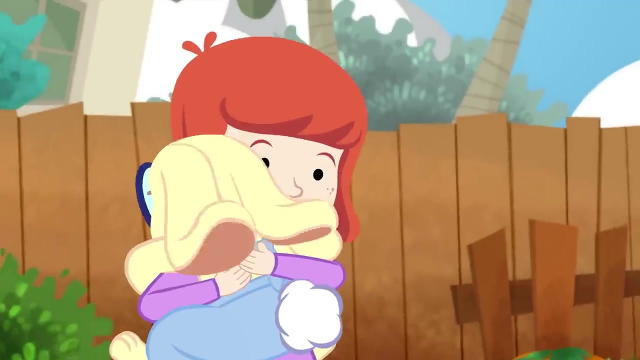 breathe. that's right, Nina. so plants are very important to all of us because they make clean air for us to breathe, and we're important to plants, too, because they need the air we breathe out to make food. yes, smarty pants, just like how. you need me and I need you. 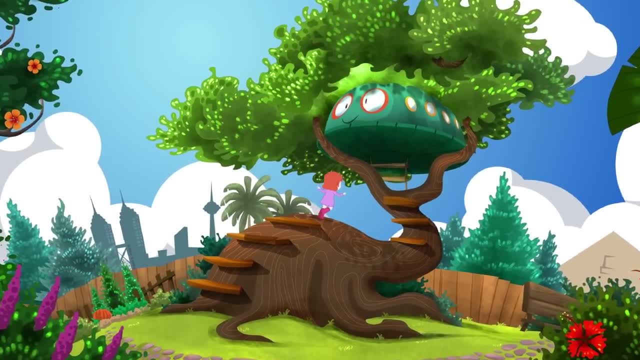 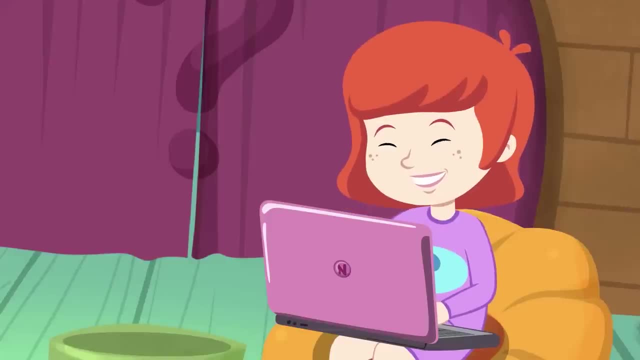